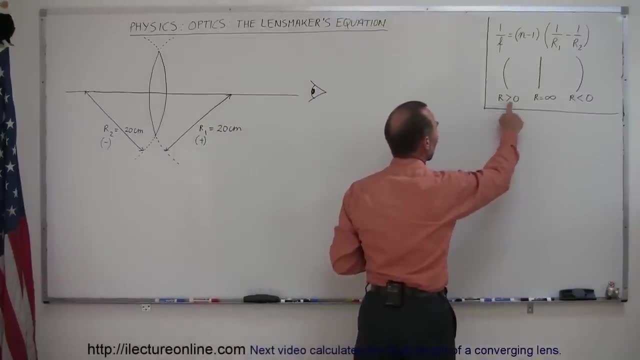 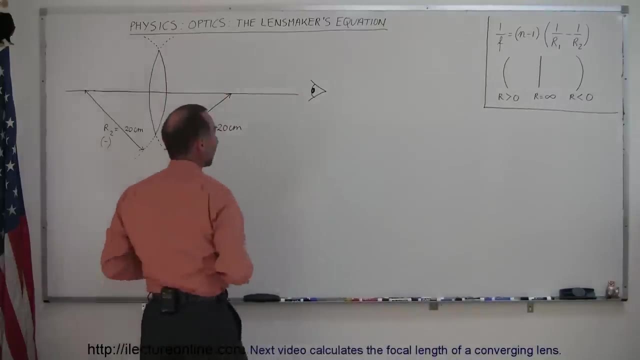 lens, and so we call the radius of curvature positive greater than zero. if the radius curvature is greater than zero, So we call the radius of curvature positive greater than zero. curves away from the observer or towards the left. If the radius of curvature bulges to the right. 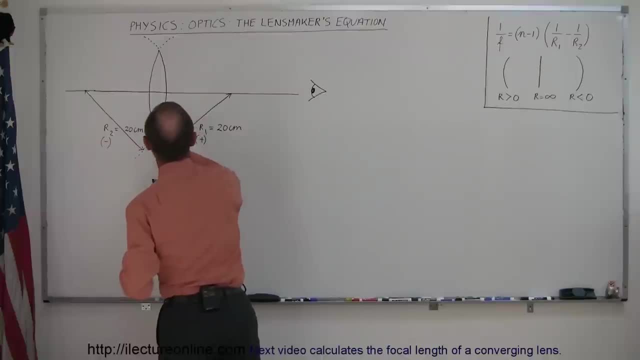 towards the observer. we call that- excuse me, we call that a positive, I'm sorry, we call that a negative- radius of curvature. So, like this, this would be negative radius of curvature. And finally, if there's no radius of curvature, if the surface is flat, then we have the radius of curvature equal. 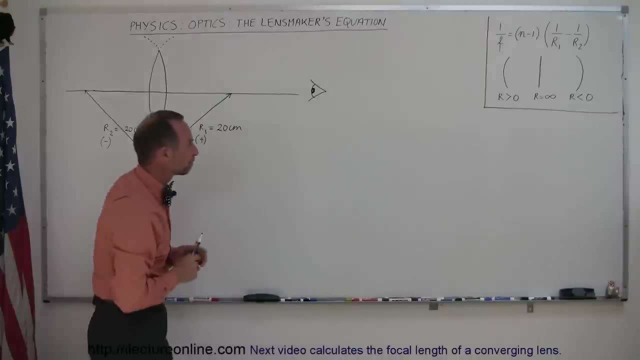 to infinity, Excuse me? Alright. so now the objective is to find the focal length of this particular lens, and let's go ahead and try to figure that out. So we use our lens makers equation. We say that 1 over the focal length is equal to n minus 1 times 1 over r1 minus 1 over r2.. Now let's say that the 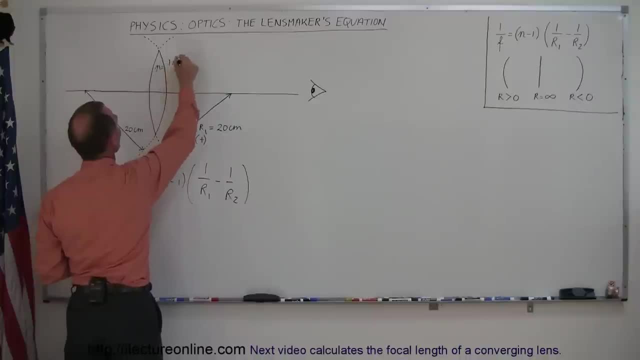 index of refraction of the glass is 1.5.. The index of refraction of the air n equals 1.. And r1 is the radius of curvature of the front of the lens and since the curvature is to the left away, 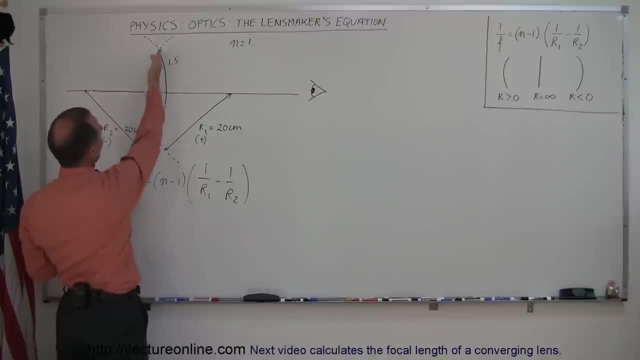 from the observer. that will be a positive quantity And you can see here that's a curvature, the center of curvature right there. So that would be a positive 20 centimeters. Let's say that the curvature of the second part of the lens, the backside of the lens, right here it bulges towards the observer. 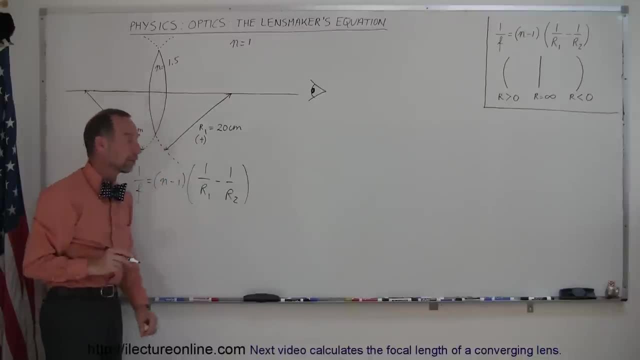 So we call that negative 20 centimeters for the radius of curvature. Plug it in the numbers we get: 1 over f Is equal to 1.5 minus 1 times 1 over r1.. r1 is a positive 20 centimeters minus 1 over r2 and r2. 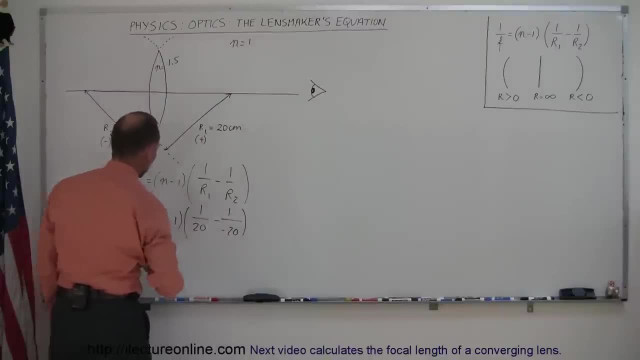 is a negative 20 centimeters. Simplifying this we get: 1 over f is equal to 1.5. minus 1 is 0.5 times 1 over 20.. Minus times the minus becomes a plus 1 over 20..